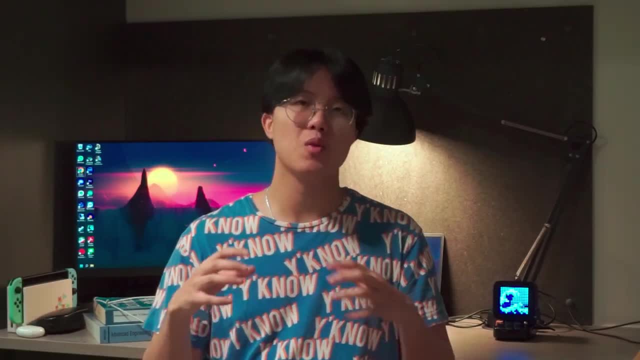 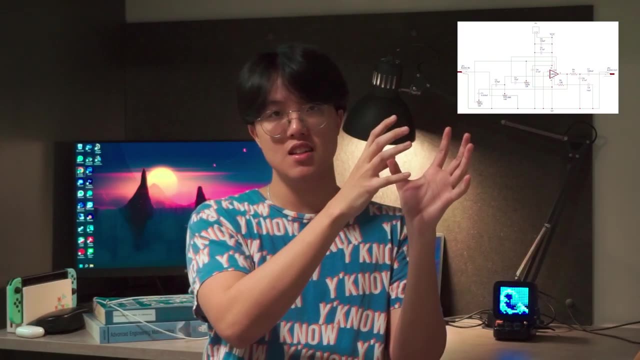 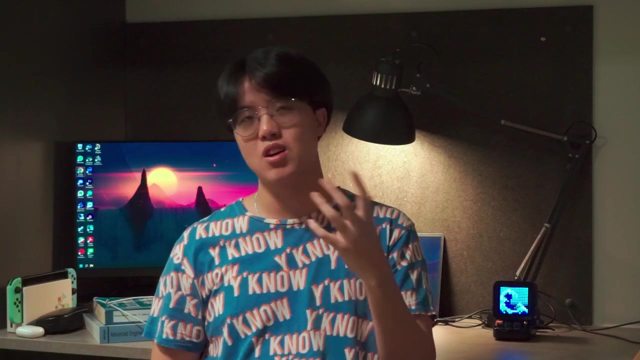 engineer if you cannot make things come to life. So what is PCB design? Well, PCB design is turning your ideas from your schematic sheet, like these, into a rectangular board like these. How do you do this? Well, you use a software, and, from my experience, what I use is Altium Designer, and that's what my 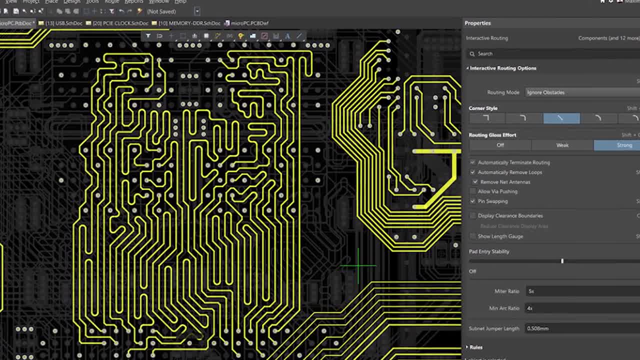 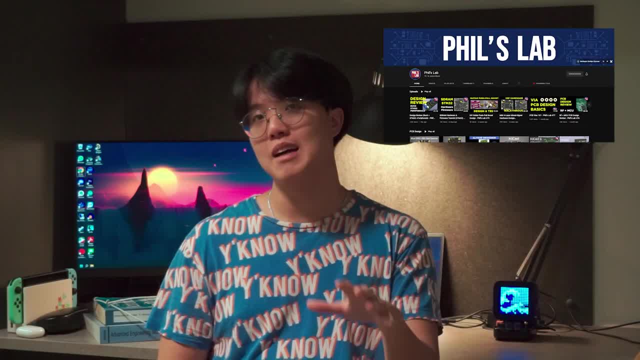 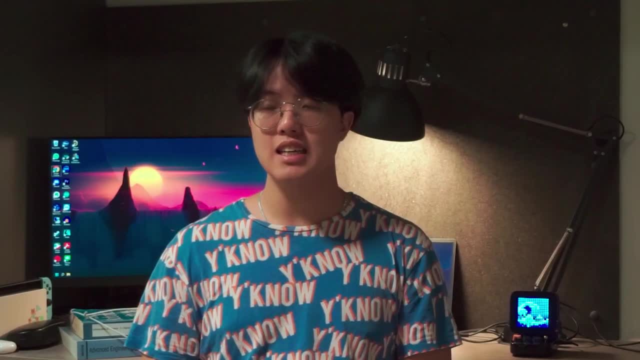 company used and that's what how I designed my board. If you're interested in learning PCB design, I would definitely recommend a YouTube channel called ThePhilzLab and he has some excellent teaching videos about PCB design. overall, He is my go-to teacher. I'll link his YouTube channel down. 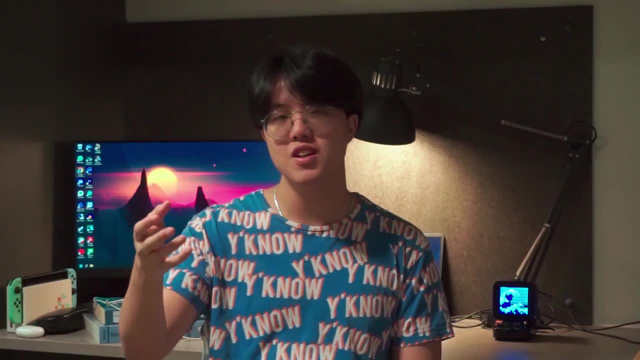 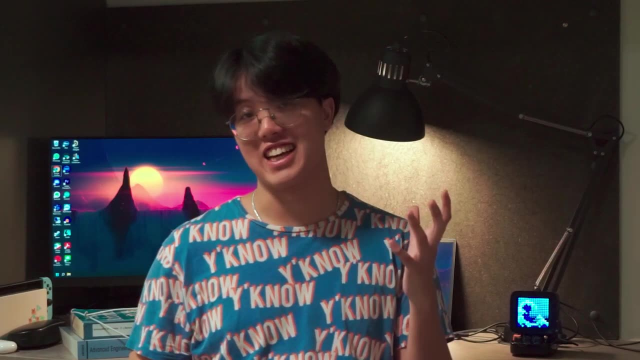 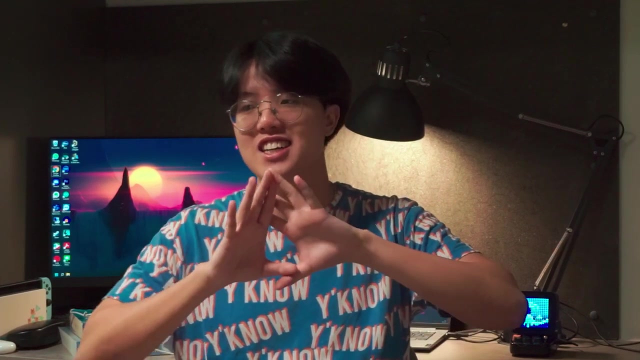 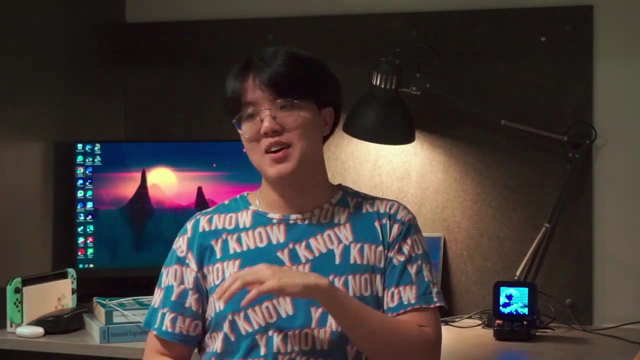 below Third skills that you can differentiate yourself with other engineers is coding. Wait, wait, I know what you're thinking. You're thinking: man, fuck coding. I hate that shit. man, Like you have avoided this entire uni life where you're basically choosing all the modules not relating to coding. Well, I want to tell. 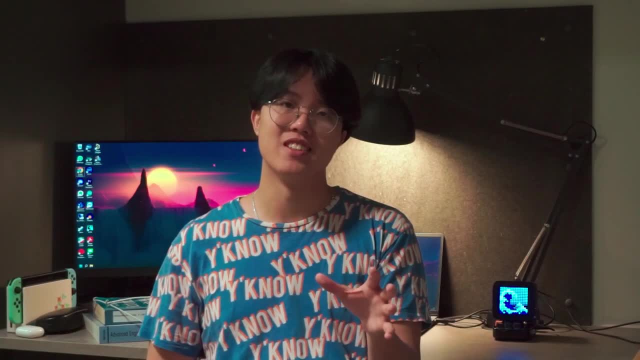 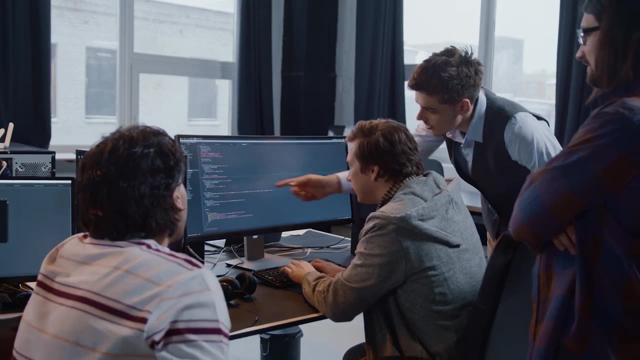 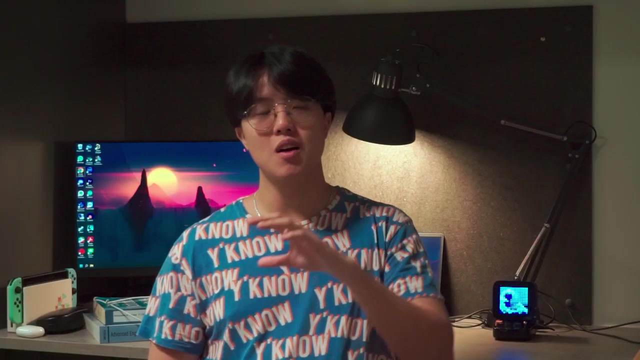 you this straight up: You cannot escape coding forever, because it will eventually catch up to you, like it did to me, And you know what I believe. I believe soon coding will be one of the main subject in school, Where it's just like math or English, and will come eventually in a world where coding will be a requirement in all schools. 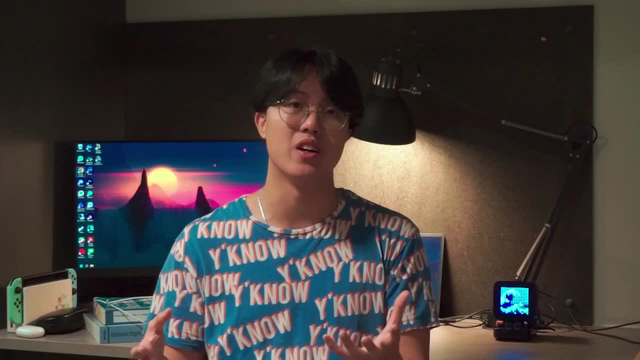 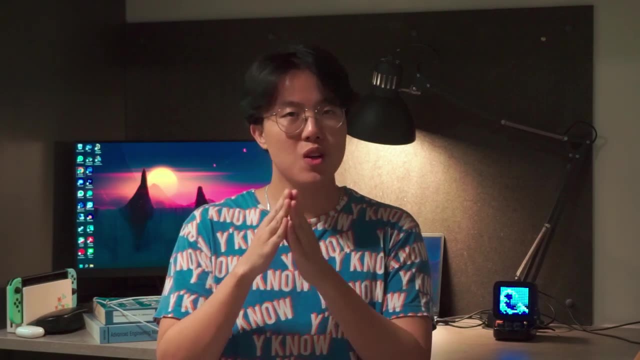 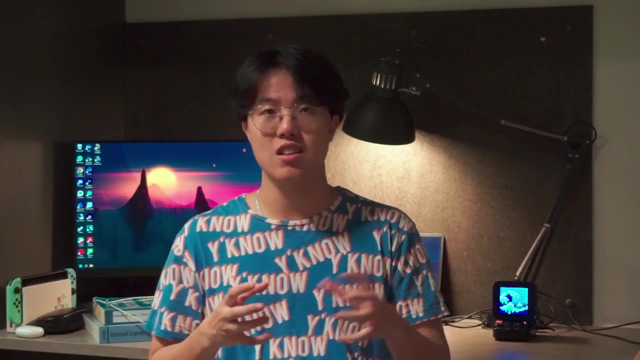 Because it is so essential. nowadays It's everywhere and anywhere, So the earlier you start, the better. Here are my suggestions. If you had only and only one choice to learn a language, I would definitely choose Python. Why? Well, Python has a lot of resources out there to learn and it's one of the 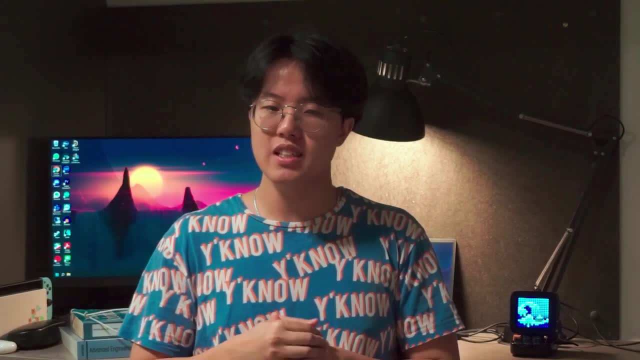 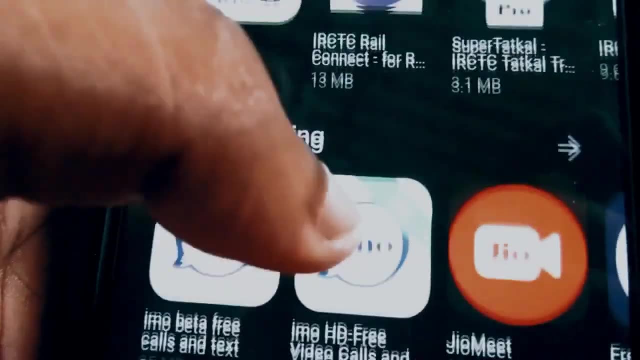 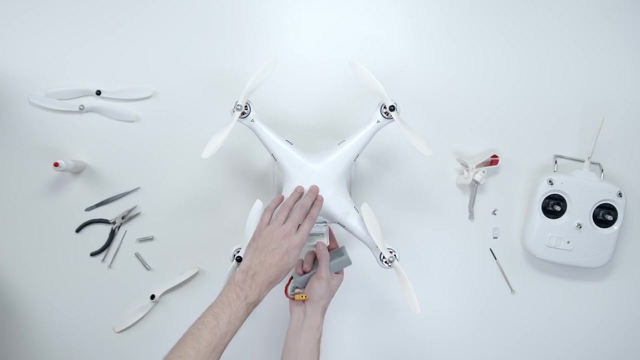 highest level languages, where it is just relatively easier to learn than other languages. And the other thing is that it's versatile. Versatile in the sense that it's applied everywhere. Just look at it: Data, AI, even now, to electronics, Literally everything. Third is that it's relatively easier. 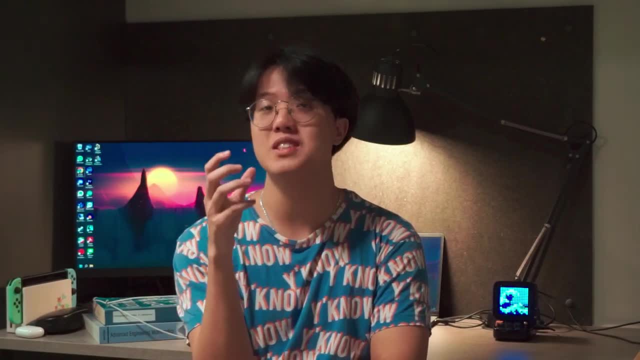 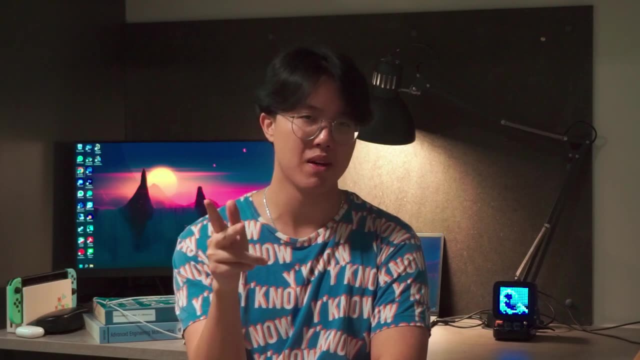 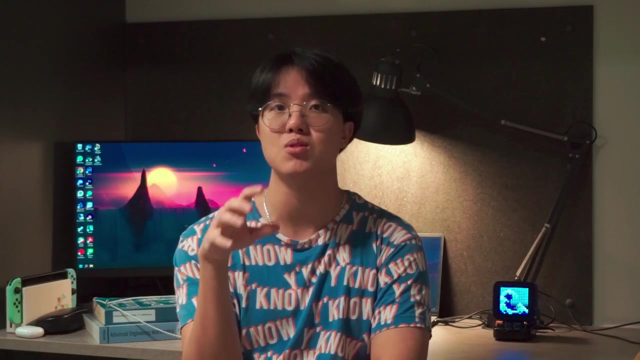 to learn than other languages out there. But if you really want to dive into electronic side of programming, I would recommend you to learn C, C++ for embedded Verilog and VHDL for FPGAs and ASIC design If you're really keen on, you know, diving into lower level programming Now that we've gone past. 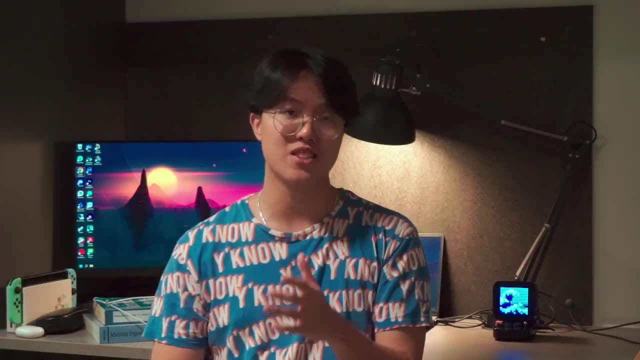 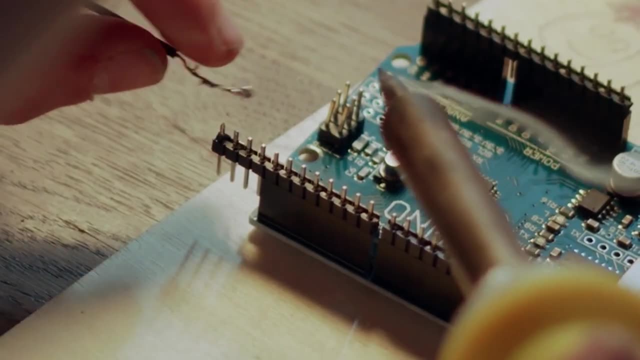 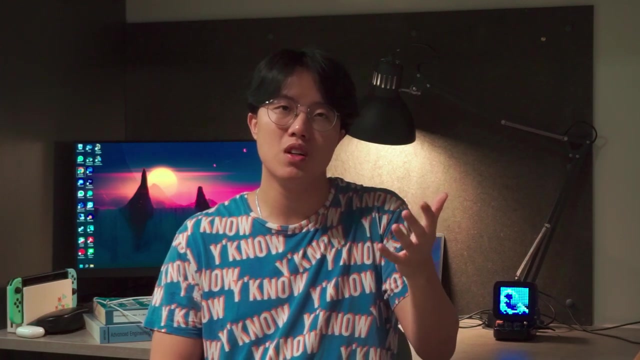 to the hard skills, let's not forget the soft skills as well. What I believe? sometimes the soft skills are even more important than the technical skills one possesses. Why do I say this? Well, anybody can learn and improve Your technical skills Just by practicing and repeating tasks. you'll eventually pick up those. 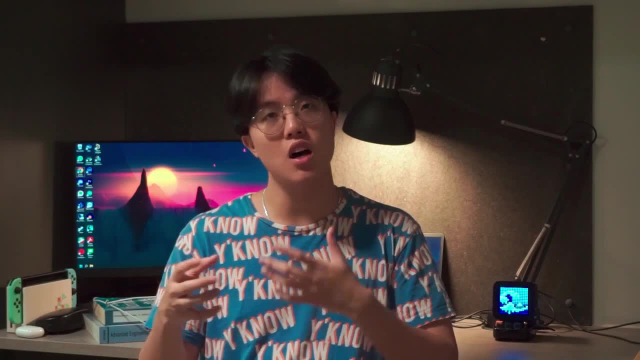 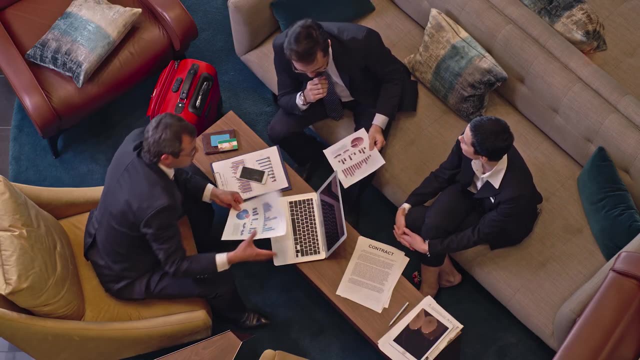 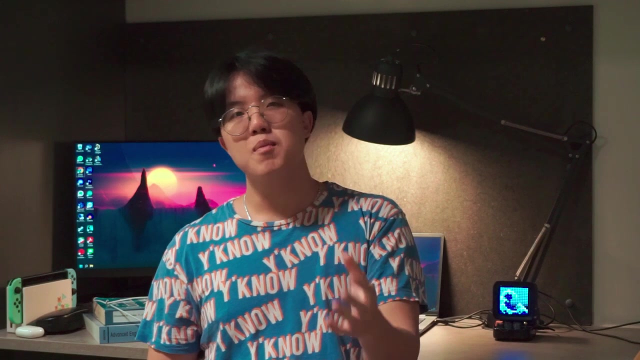 things. But what's harder to change, harder to pick up, is your thinking and your mindset. The first soft skills is learning how to communicate your design and your ideas clearly to other people. This is so crucial is because if you're unable to communicate your ideas clearly, you will not move. 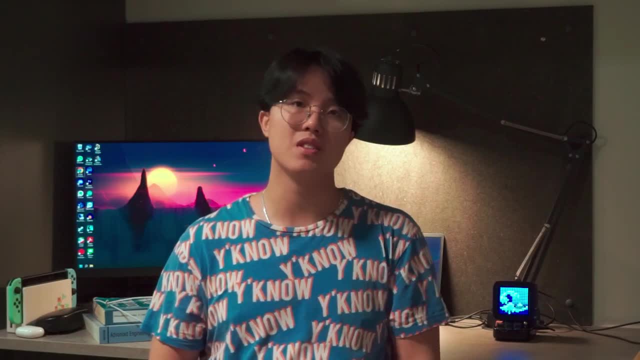 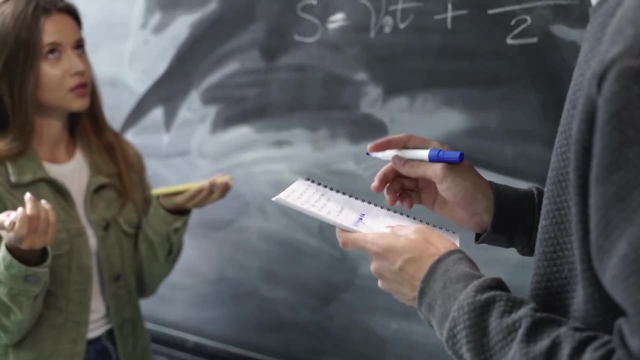 far in your programming. If you're unable to communicate your ideas clearly, you will not move far in your programming, Career life, or even if you're trying to start a business or a tech startup, is because people will not take you seriously. How do you improve on this, you may ask? Well, being able to explain your ideas. 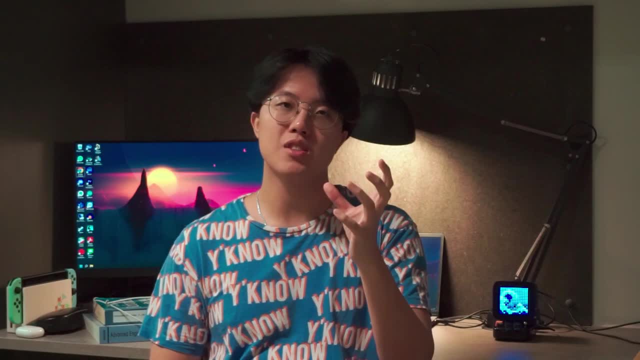 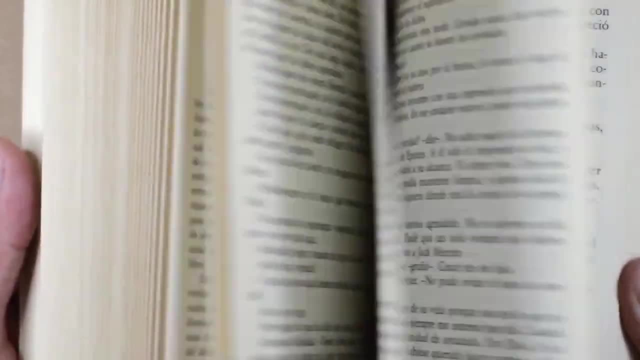 clearly comes with the depth and mastery you have in a certain topic, right? So my number one recommendation for you is to read and expand your vocabularies in that subject or whatever you're interested in. Don't be afraid to go back and polish your 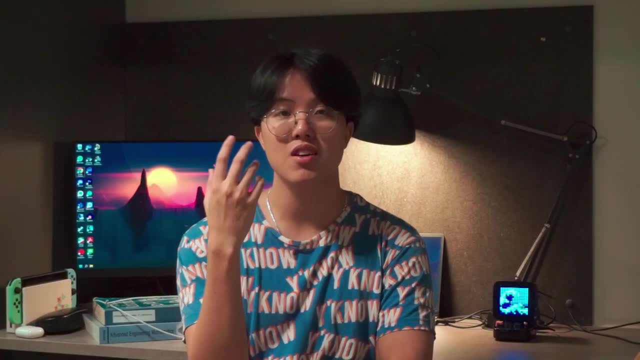 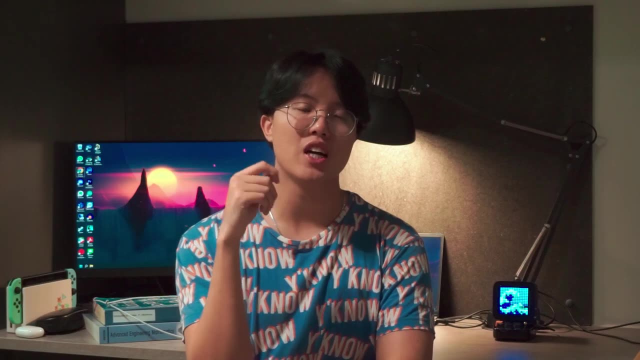 basics as well, because that's what I'm doing right now. What I've realized is that I have a lot of knowledge gaps in my fundamentals. It is really detrimental for me when I'm trying to explain something to other people is because if I don't understand the basics, how am I supposed to even 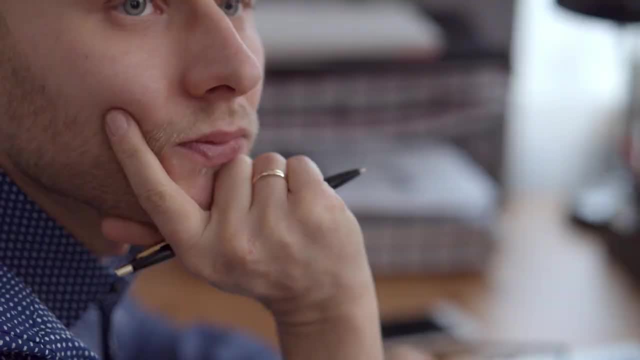 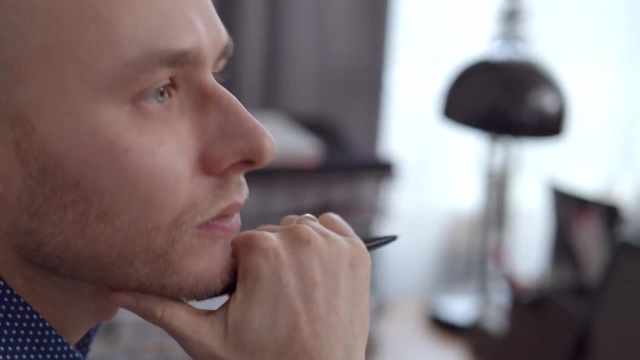 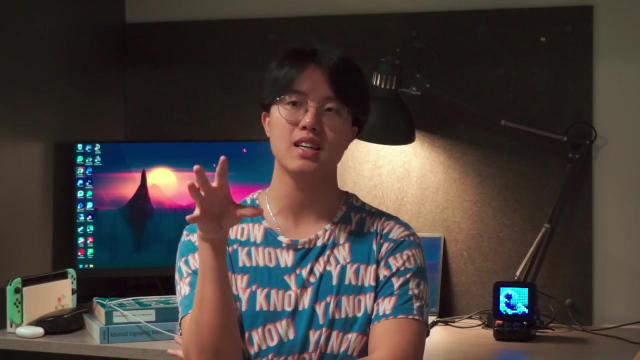 communicate a more complex idea right. Finally, you need to think like an engineer. You need to have a higher level thinking process. What I mean by this is that, for example, instead of just jumping into a project straight away, define a clear goal and set of requirements you want for.